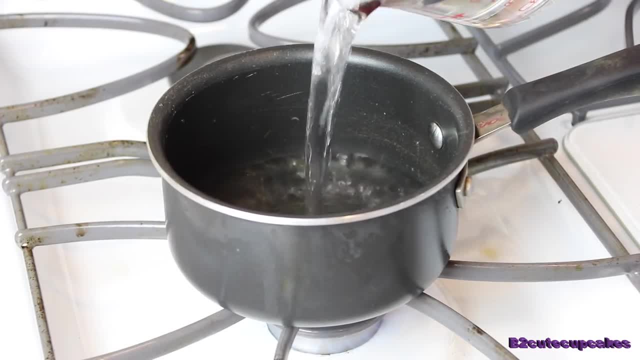 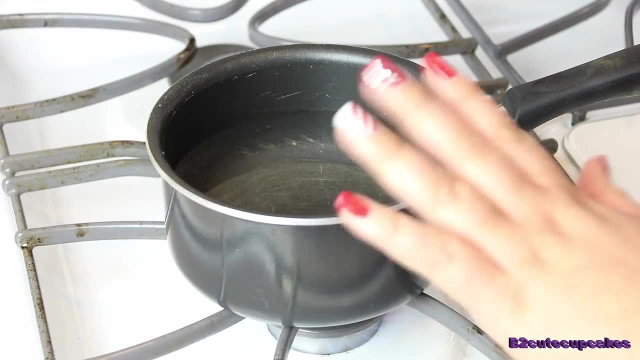 And then we need two cups of water. I'm going to pour it in There, two cups of water. Okay, so we are going to wait for a little bit until the water kind of boils a little bit, And then we're going to pour one cup of salt. 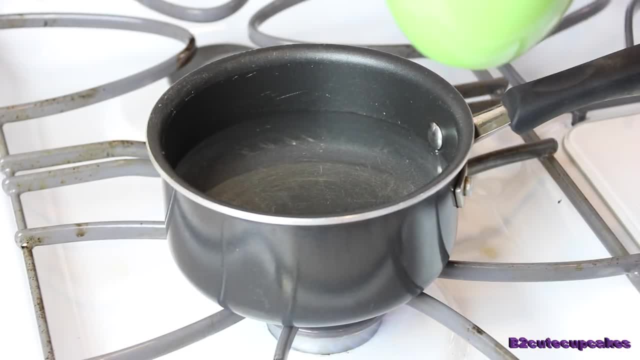 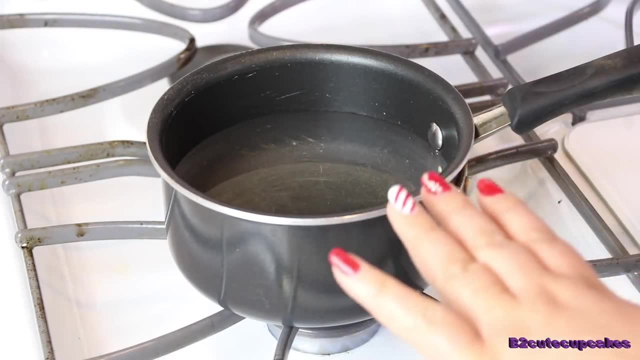 And, don't worry, I'll leave all the ingredients in the description box And the process I'll have to make it So, in case something is not clear, just go read the description box. okay, While this water boils, we're going to do something in this bowl. 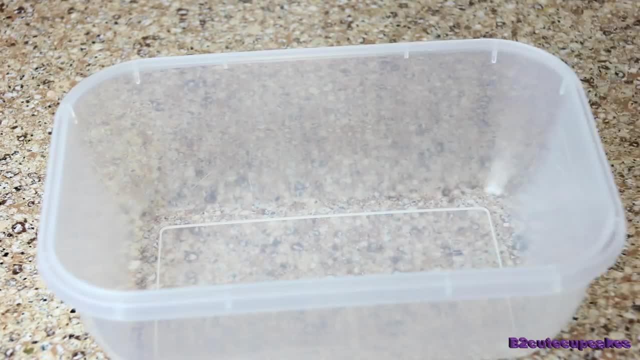 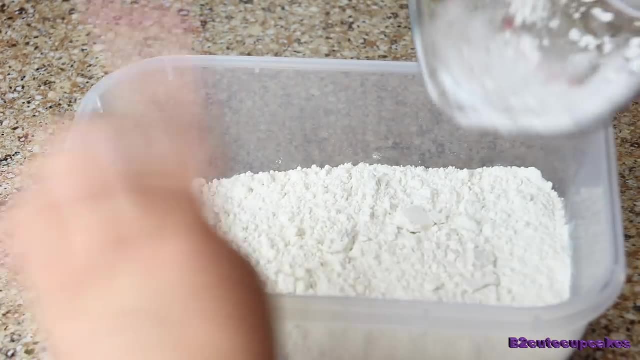 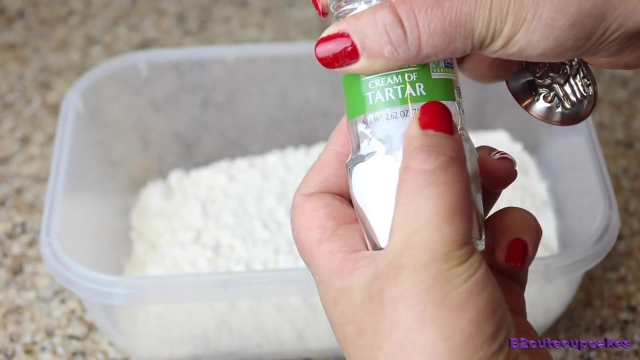 Okay, cupcakes. So right here we're going to pour two cups of just all-purpose flour, And Bia is just going to pour it in here. Alright, that's two cups of all-purpose flour, And then we're going to pour five teaspoons of cream of tartar. okay, 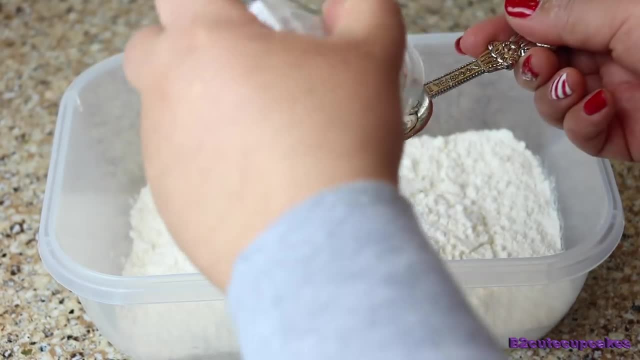 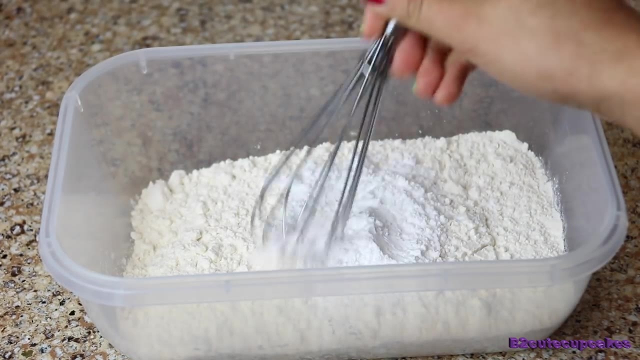 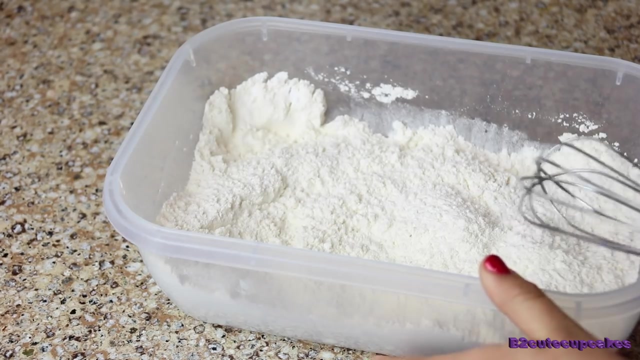 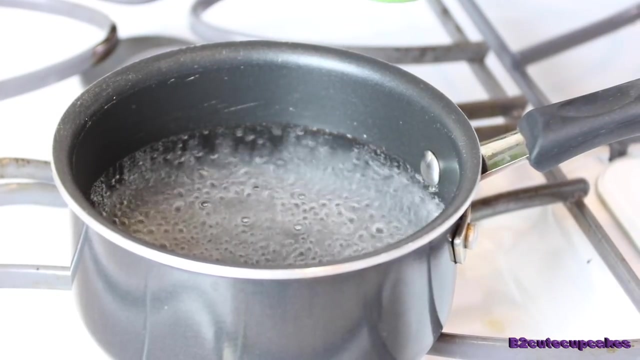 Five teaspoons. Okay, Now we're going to mix this. I'm sorry for my voice, Okay, so let's leave this here aside. Now we're going to pour one cup of salt into our two cups of water. See, the water is now boiling, so let's pour it in. 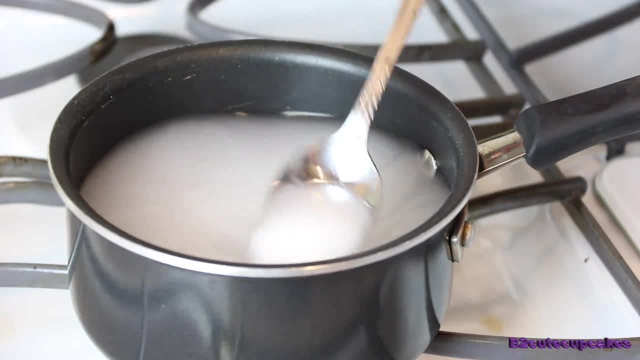 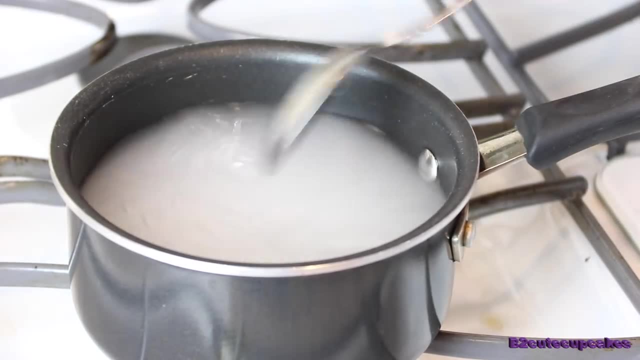 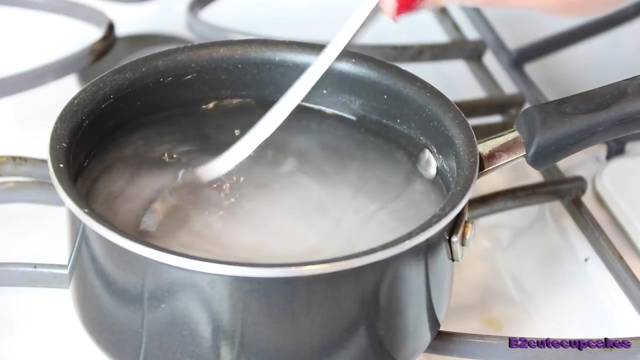 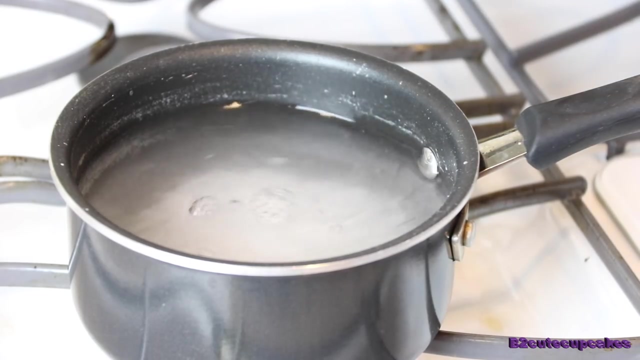 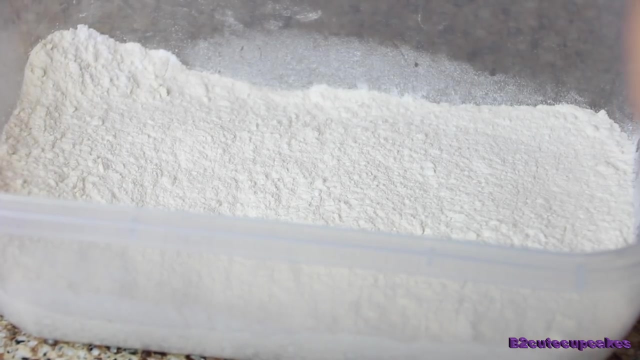 And we are going to move that just a little okay, Not too much. Okay. we're going to move our water, our salty water, again just a little, Okay, And I'm going to turn it off now. Now, into this flour, we're going to pour in two tablespoons of oil. 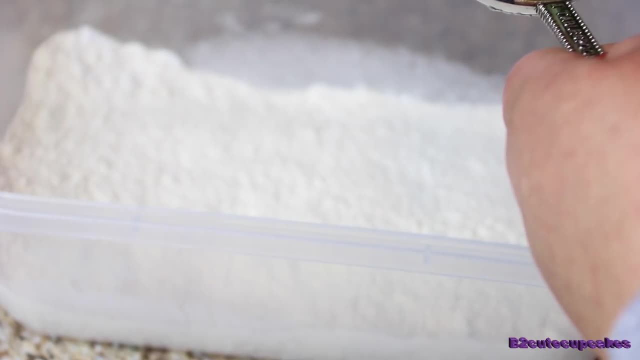 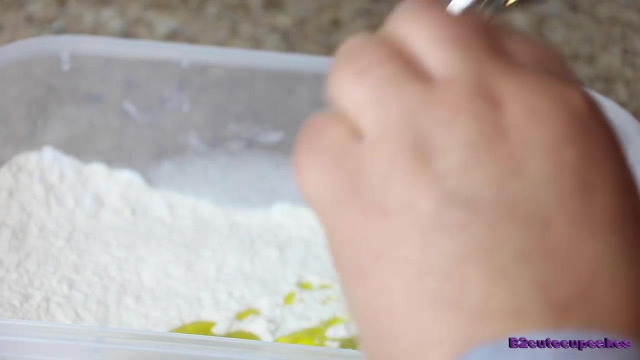 It can be any kind of oil you have. In this case, I'm using olive oil, but you can use any kind of oil you have. You can use any kind of oil you have. okay, So we're going to pour one, two tablespoons. 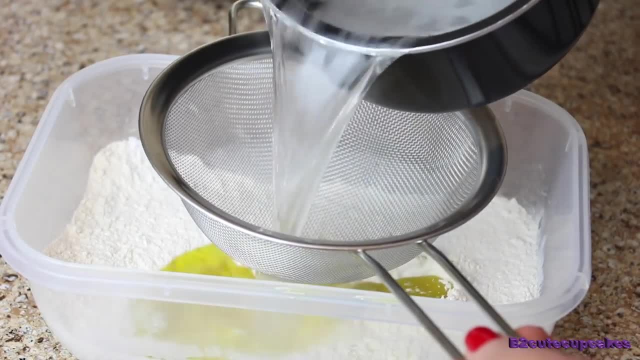 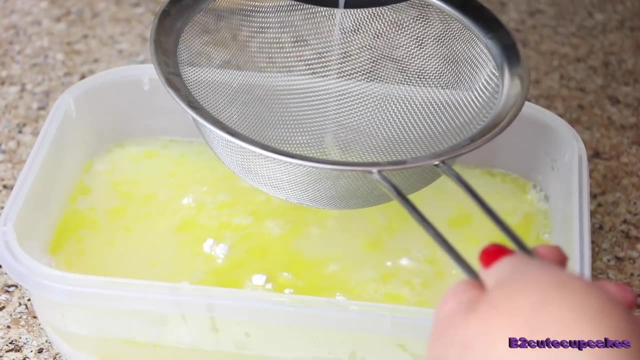 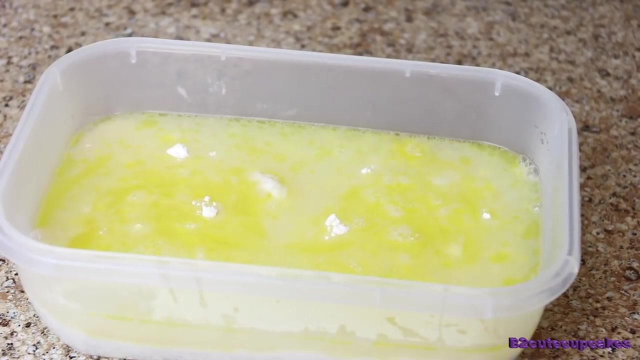 Okay, now we're just going to pour the water in here, the salt water, Or the water with salt, whatever. Just pour it in, And look at all the salt we have left. That's a lot of salt. Okay, now we're just going to mix this. 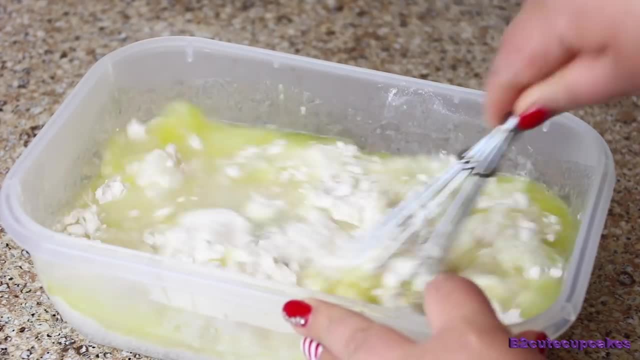 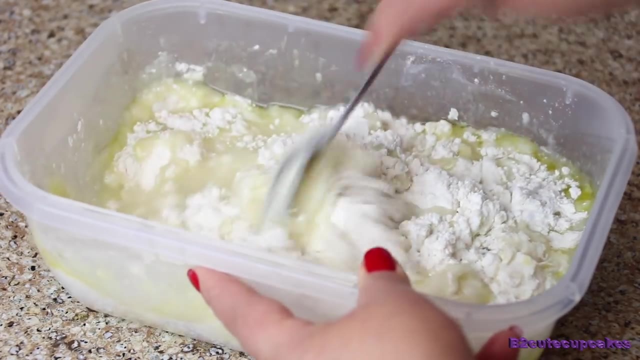 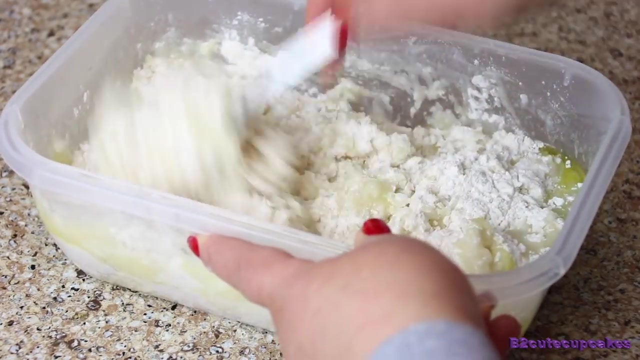 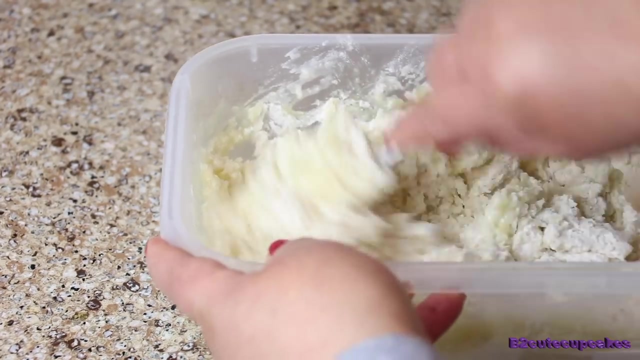 I'm going to use a spoon to do it. It's a lot easier to mix it with a spoon, And don't put your hands in there just yet, because this is hot, Extremely hot. Okay, Okay, you see. You see how it's coming together. 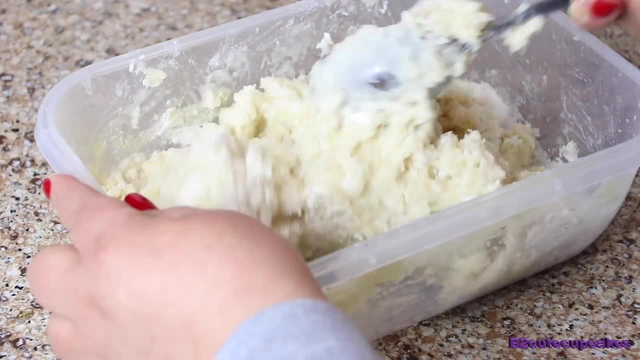 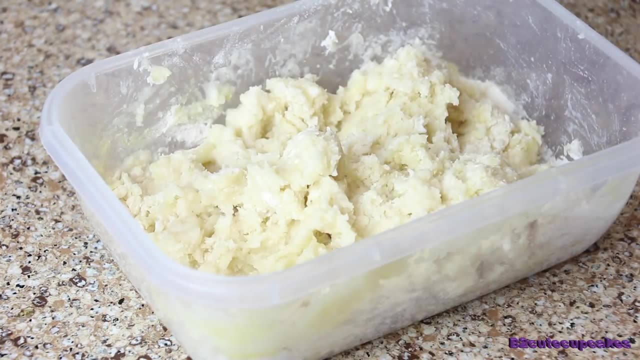 We're going to let it cool down for a little bit and then we're going to start doing it with our hands, Because right now it's still pretty hot, so you don't want to burn your hands. Just wait a little bit. 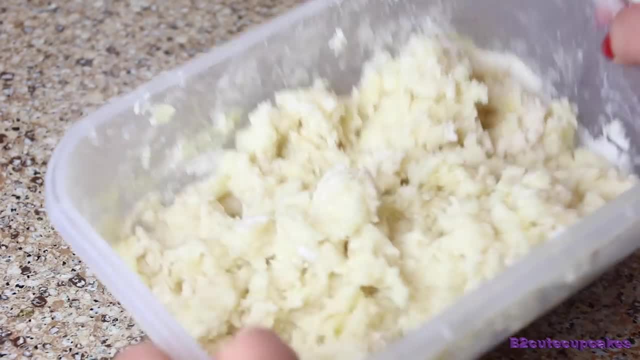 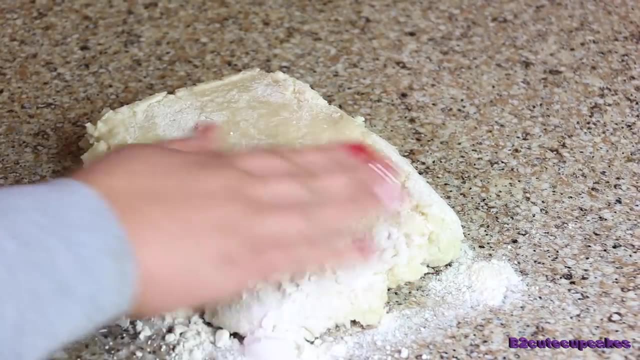 And we are going to move to another area where we can work- Okay, cupcakes. So I'm going to pour all of this here into the countertop And now I'm going to start working this with my hands. It's still pretty hot, so you can wait for about 15 minutes. 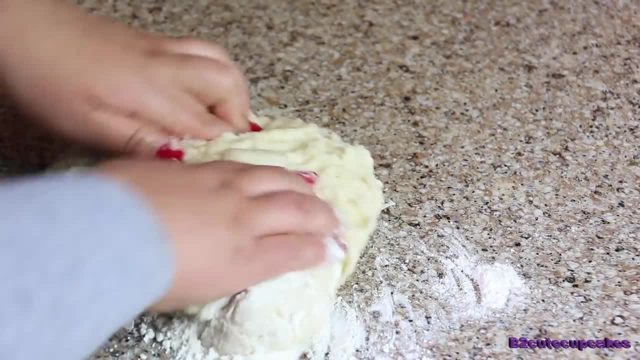 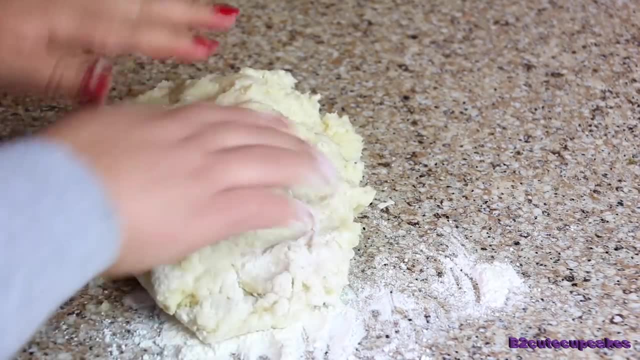 15 to 20 minutes to cool down. This one's still pretty hot because it's only been like 3 minutes, But the countertop is a little bit cool, so that'll help me a little bit And we just have to work. 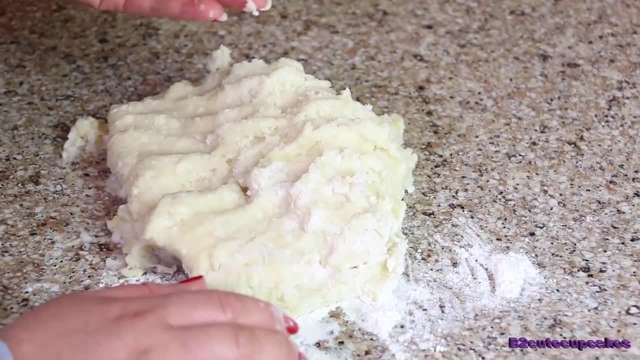 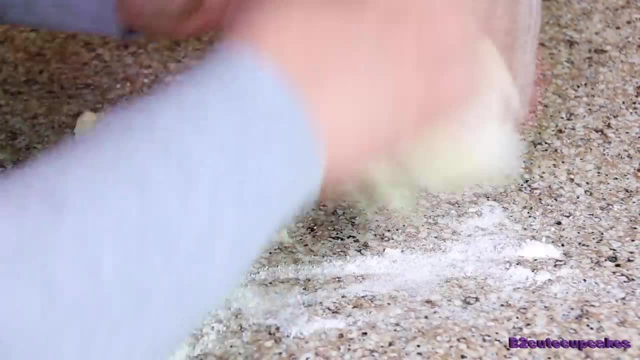 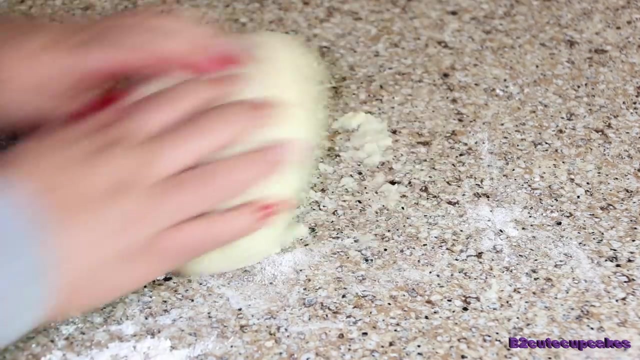 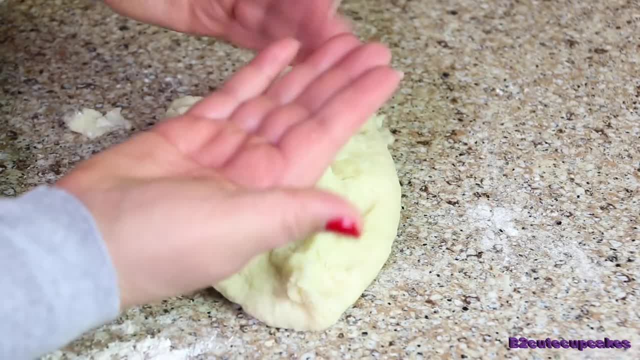 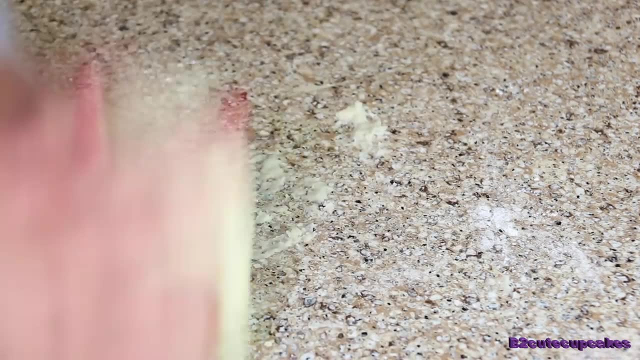 to feel it. See, right now it still have a lot of lumps and it's really hot. Look at my hands. It's like I'm burning my hands right now. That's why I'm telling you you need someone to help you make this dough. 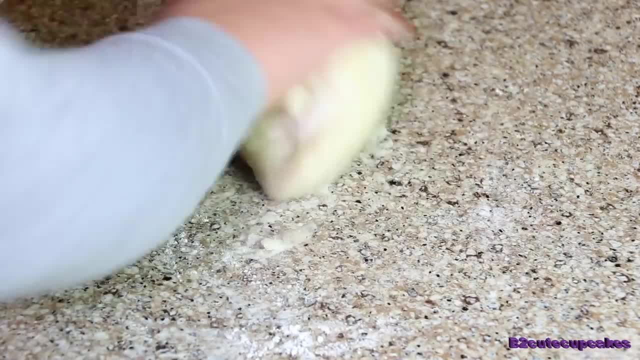 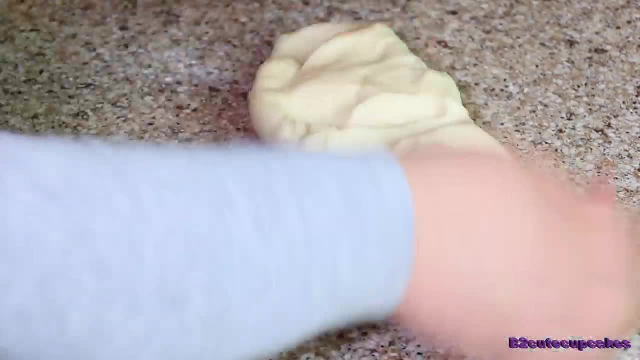 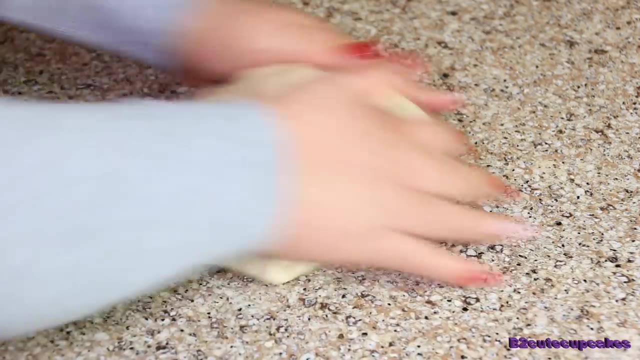 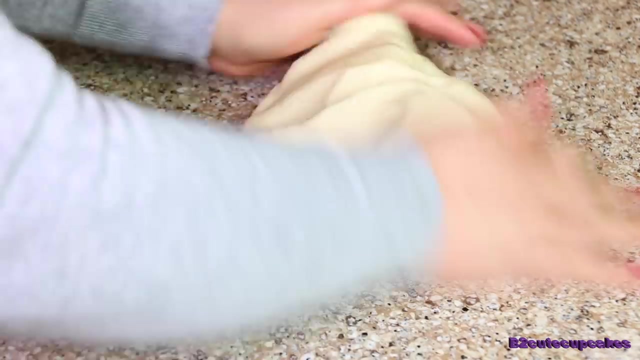 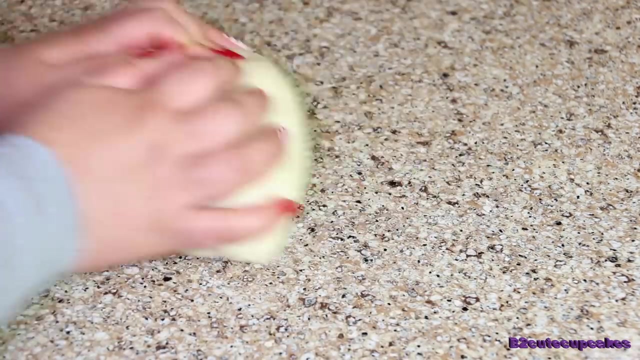 You don't do it by yourselves, because you can hurt yourself, You can burn yourself. It's getting a lot better now. You can tell right here. You see how it looks really smooth. now There's a lot of ways you can make Play-Doh, but to me this way is the best way because 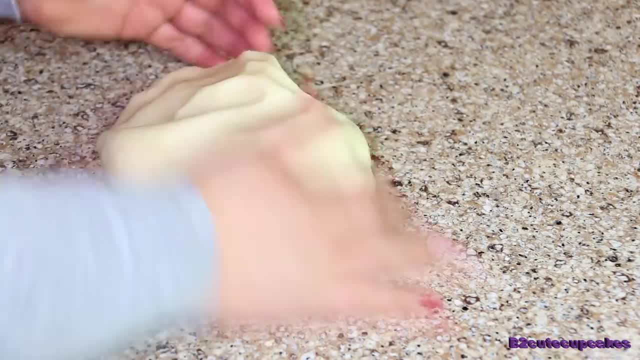 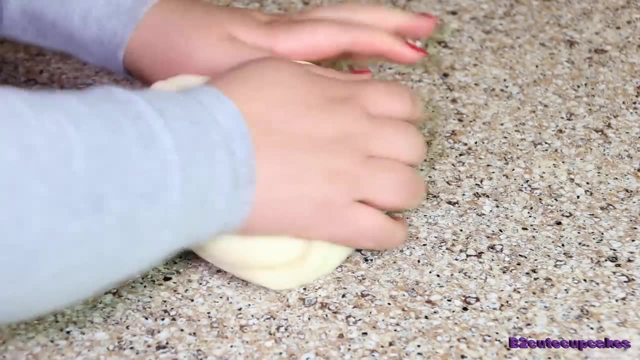 the Play-Doh lasts for a long time. Right now I'm going to show you the Play-Doh we made about a month ago or so. It's been probably three weeks since we made it and it still looks really good. The texture is still like the first day. 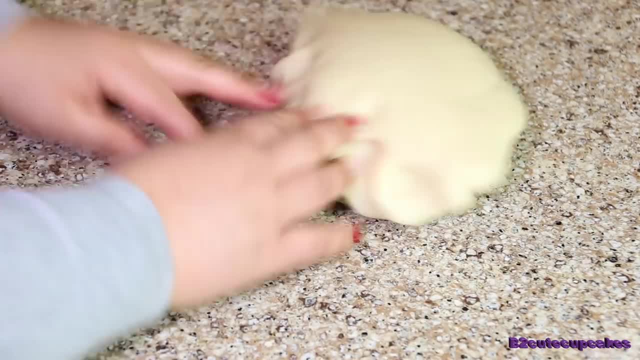 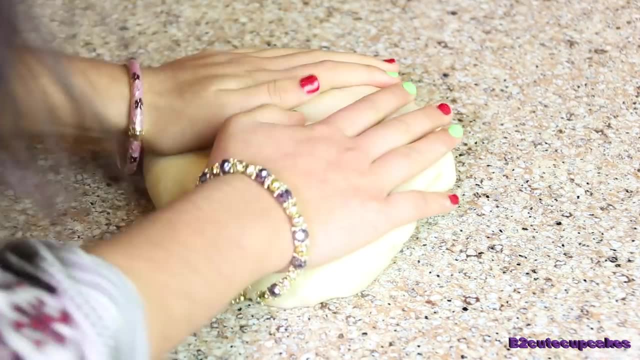 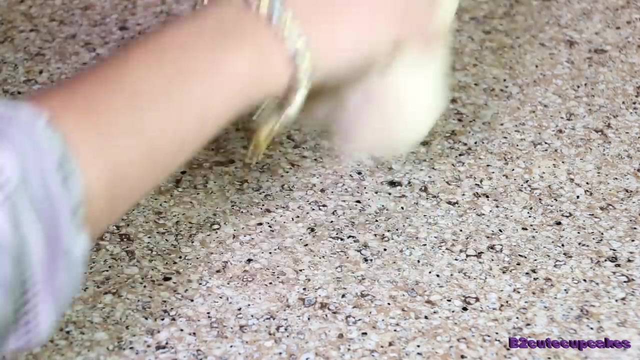 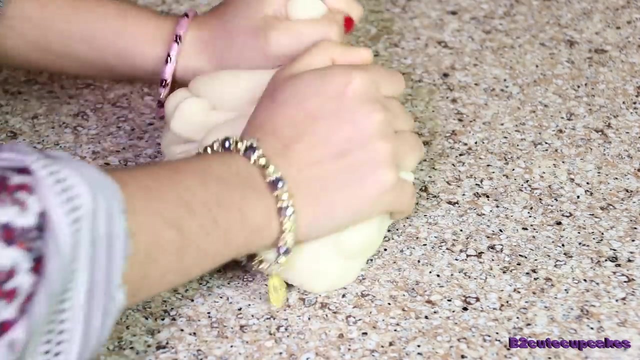 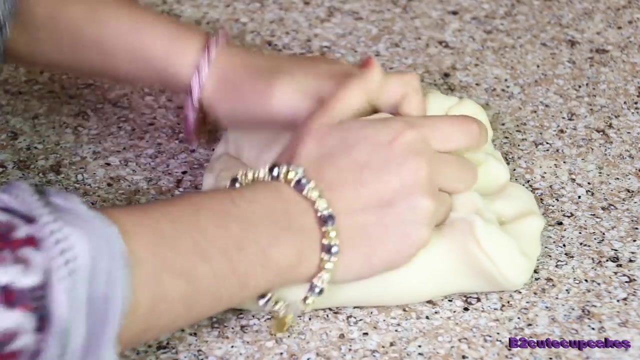 It's not dry or anything, so that's why I love it. I like this. Okay, now Bea is going to work the dog for a little bit so she can just play with it. It's warm, huh, Very hot, Okay. so now we're going to paint the dog. 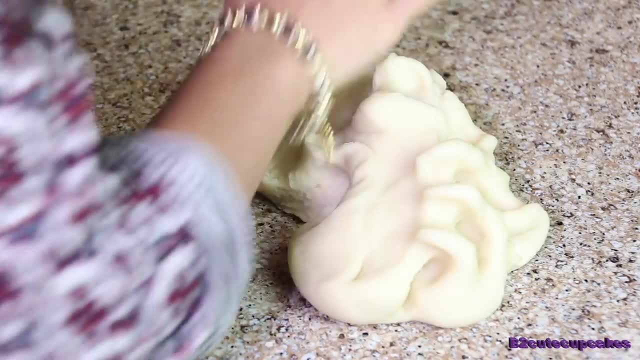 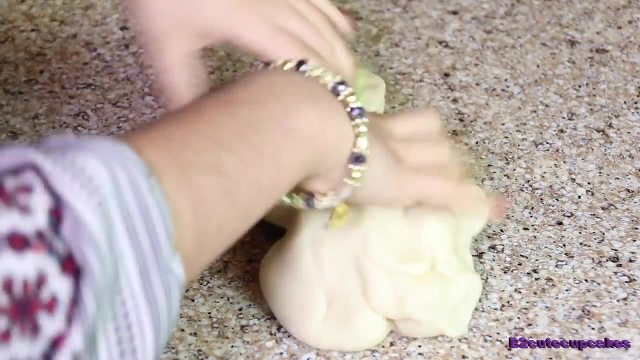 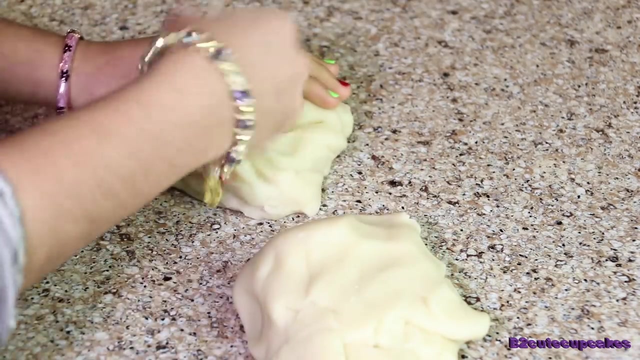 We're going to paint our Play-Doh and Bea. why don't you pick the colors? What colors do you want to make? Blue and yellow, Blue and yellow. Okay, so we're going to cut it in half. I think you need to put more over here. 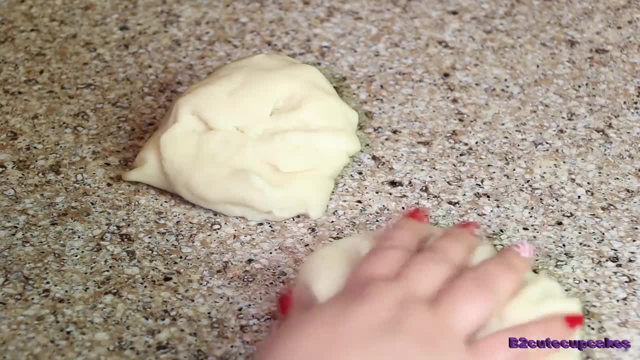 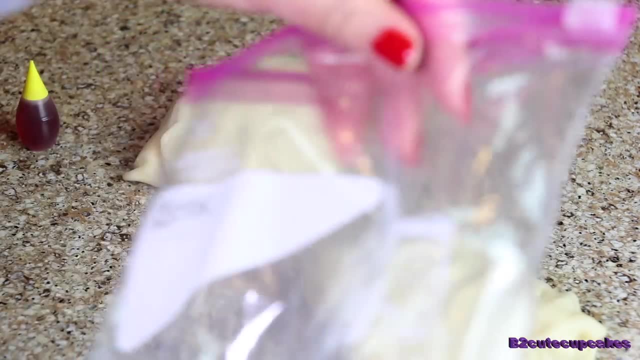 There you go. That's about half, so why don't you? I make blue and you make yellow, Okay, Okay, but this is how we're going to do it. You're going to need two of these Ziploc Zippy bags, you know, Ziploc bags. 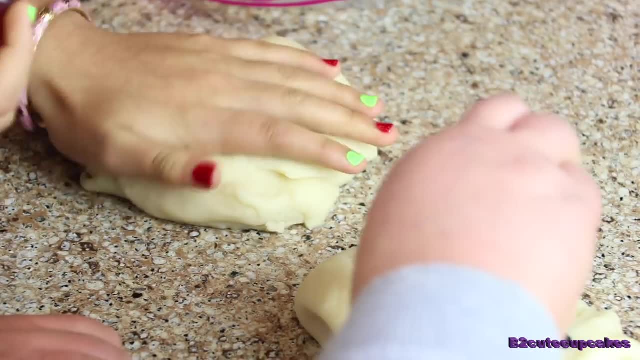 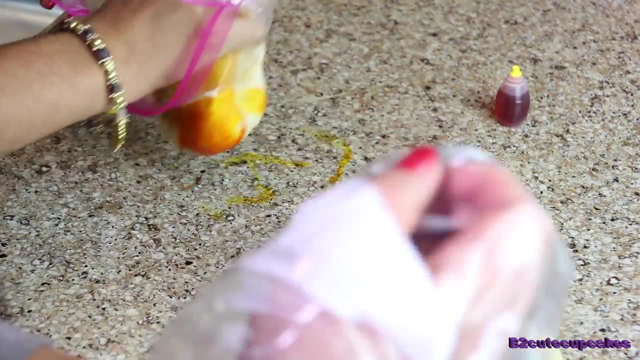 So we're going to need two and you're just going to pour in the food coloring, Just going to pour in like ten drops. Okay, so these bags, you turn them inside out and then you put your hand in there and then you start working your dog. 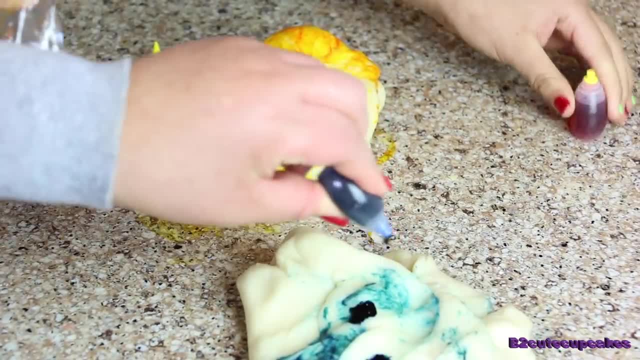 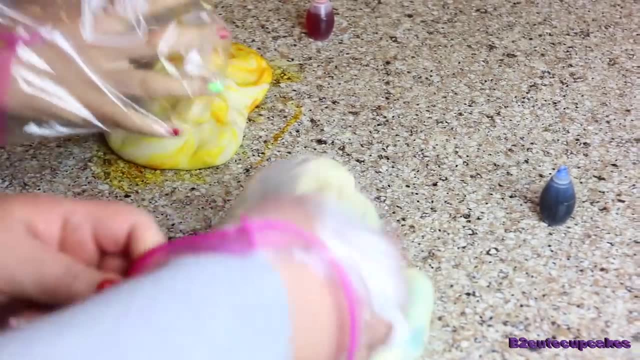 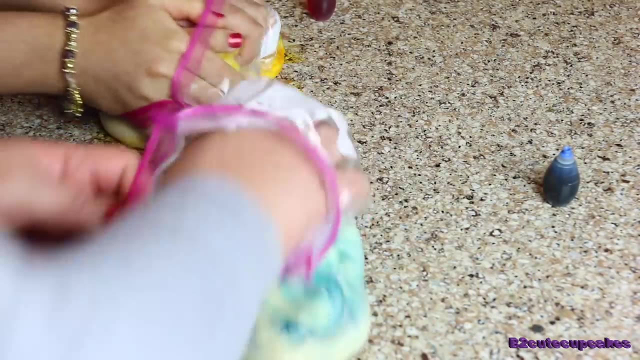 I'm going to put in more food coloring. You see how Bea pour in. oh wow, that looks cute. Alright, You can do it straight with your hands too, but then, remember, your hands are going to be blue for a couple days. I don't want that. it leaves me. 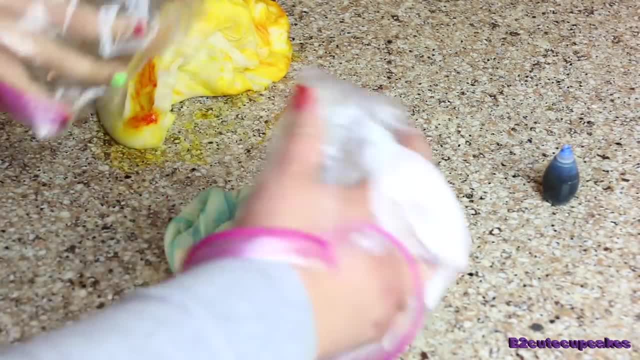 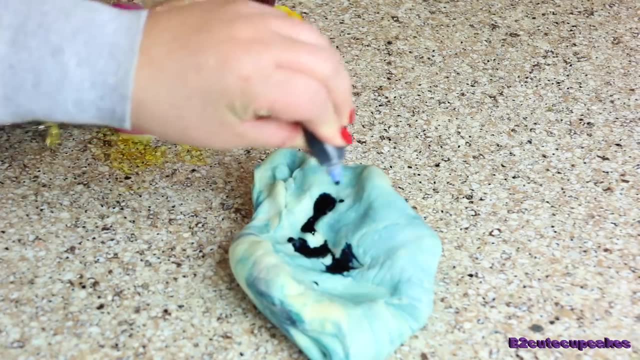 Oh, another tip that I want to give you. I mean, we have a quick tip for you, and that tip is that if you can find the- Okay, If you can find the gel- I think it's called gel painting- The gel food coloring is way better, because this is food coloring. and if you find the, 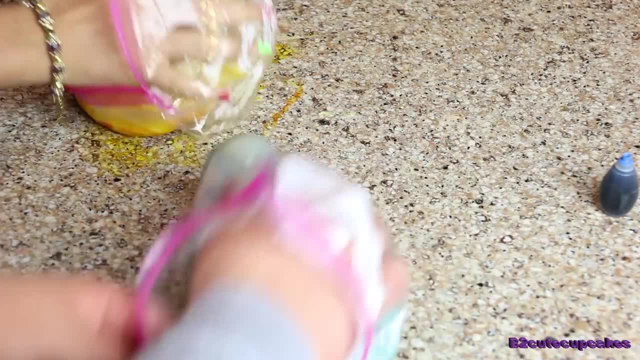 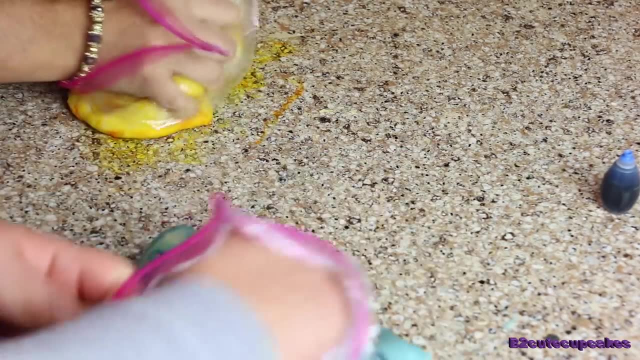 one that is not liquid but it's like a little pasty. that's better. Why is it better? Because you only need one drop of that one. Bea is asking me why it's better. It's better because that kind of food coloring- you only need one or two drops and that's. 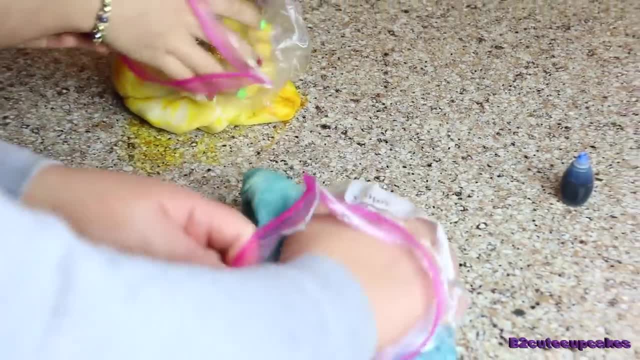 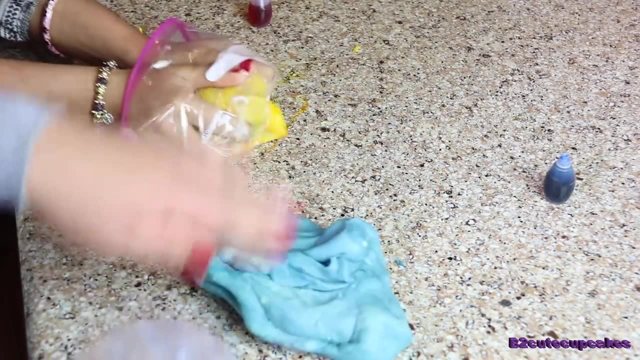 all you need A little goes a long way, And that's it. It goes a long way. And this one you have to pour in a lot. See, right here it's kind of a light blue. We can leave it like that or we can keep adding more color if we want it like a dark blue. 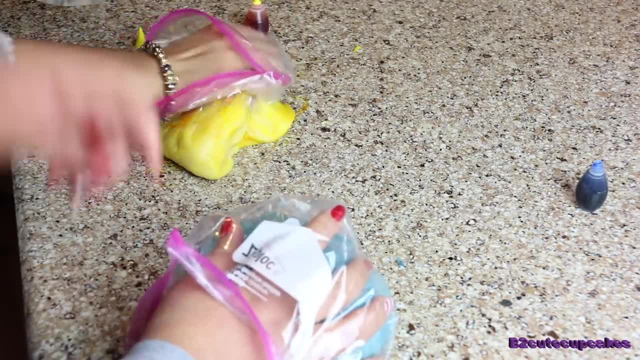 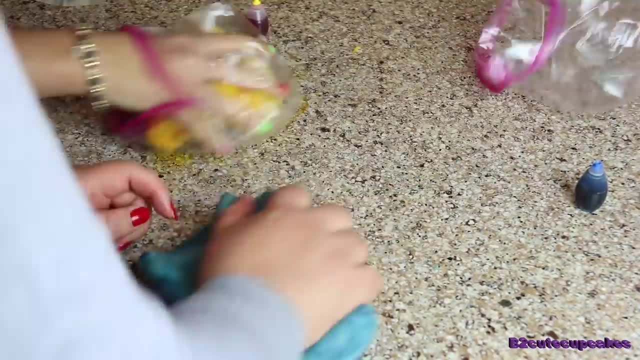 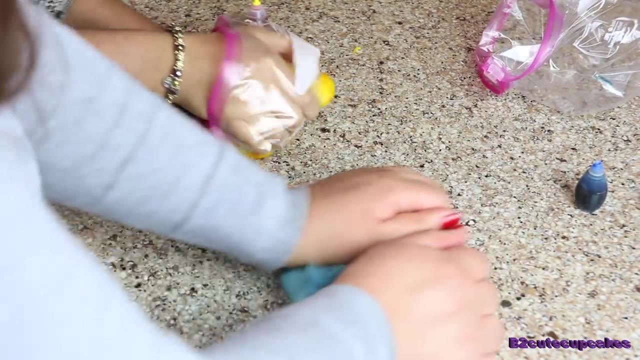 Look how cute that one is. Show them. Oh, that's so cute. Okay, now I can work it with my hands. Oh, this is so much fun. This is so much fun to work with guys. It's just like, ahh, it feels so soft. 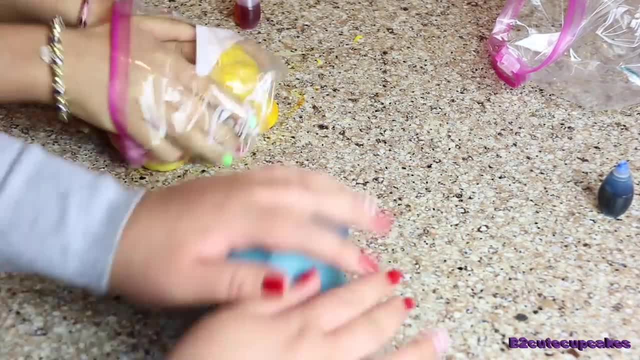 Let us know in the comments if you guys make this recipe. okay, If you guys make this DIY, because you guys are going to love it, I'm telling you You guys are going to love it so much. It looks really pretty. Show them your color. 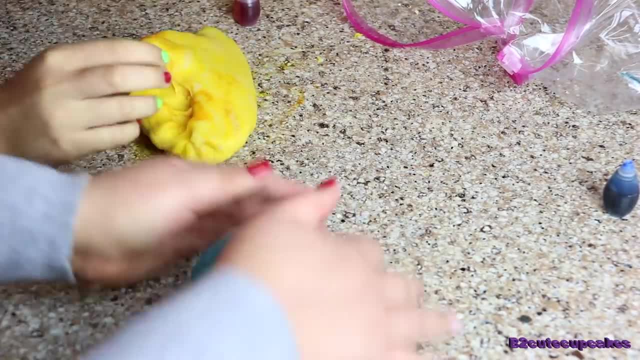 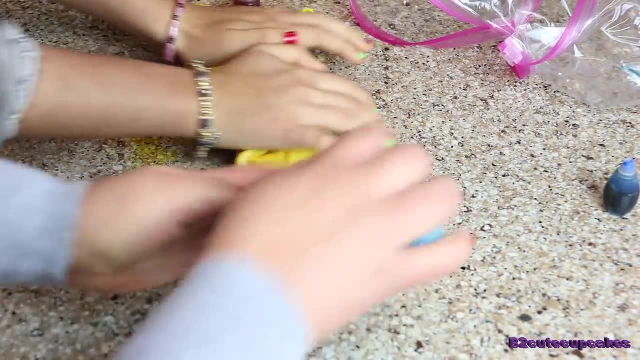 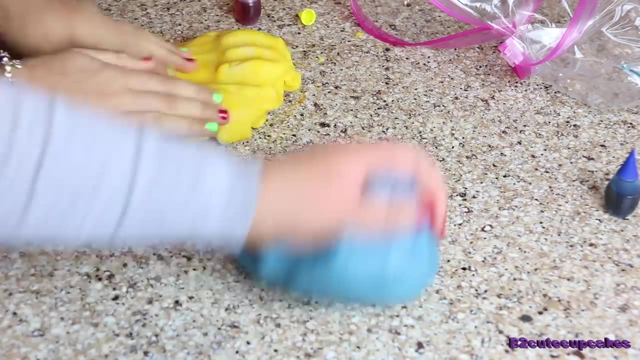 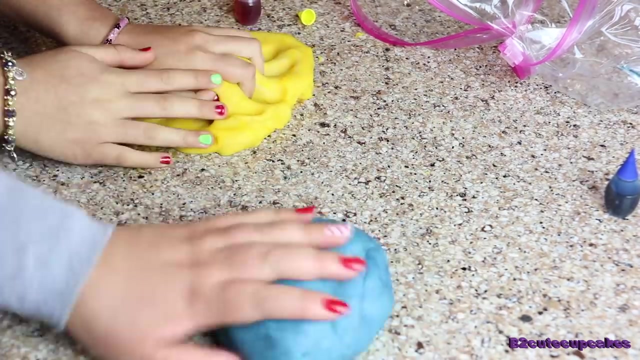 I think they haven't seen that one. Look at that one. Oh, that one looks better than mine actually. Okay, see, Now here we have a lot of blue playdoh And it's going to be good for months. Look. 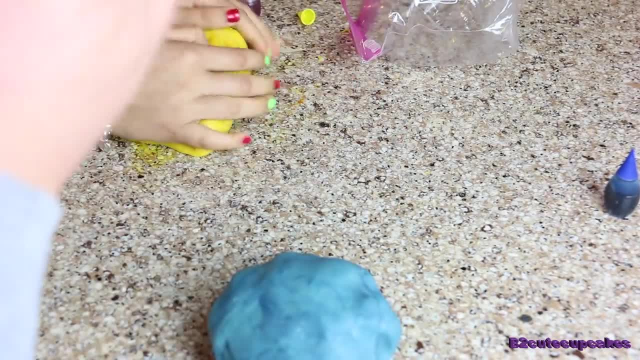 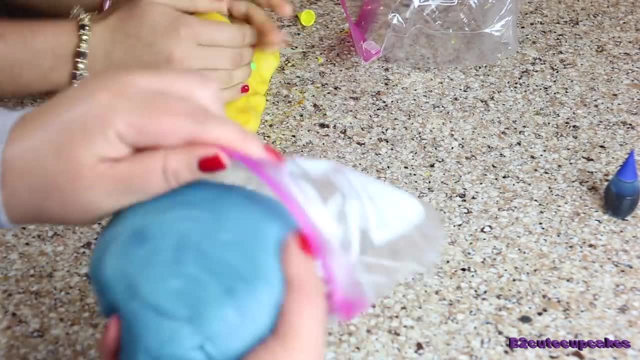 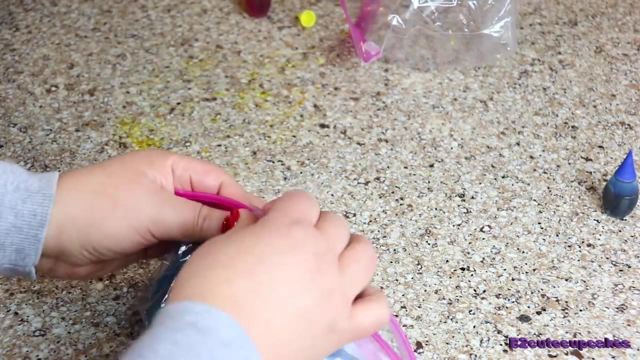 And then when you're done- I mean you can play with it and do whatever you want to do- And then you just go ahead and put your playdoh- when you're done playing or doing whatever you're going to do- Put it on your little baggie and then you just take all the air out and close it. 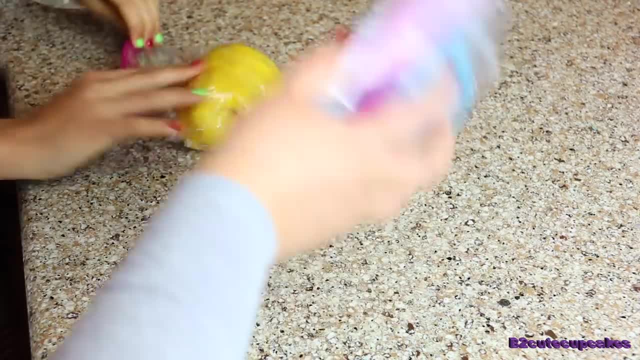 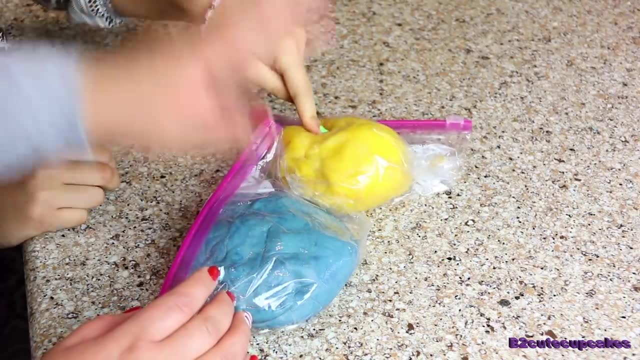 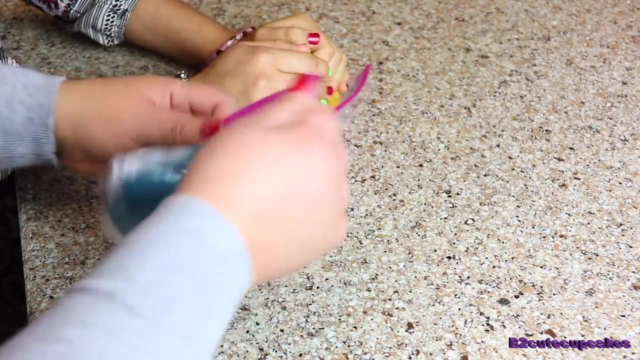 Slip it and there you go. There you have it. So now we have two playdoh colors. If you want a lot of playdoh, the same color you can just put in the food coloring, and then the whole dough base that we show you. 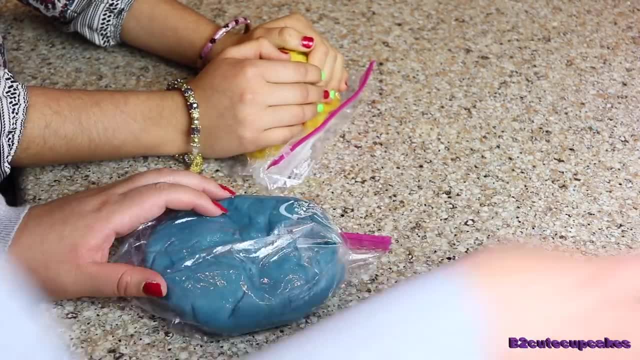 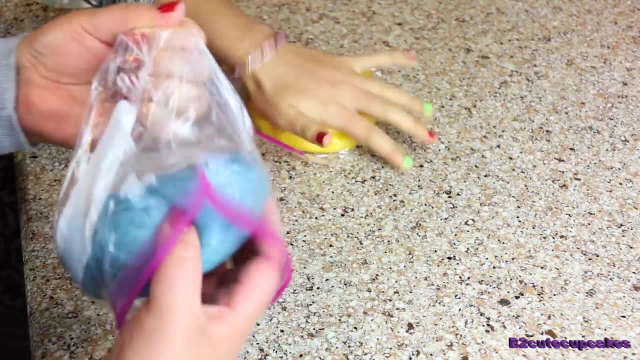 But you can even divide this into little balls and make them all different colors. That's up to you. We just want to show you how to make two colors, okay, Okay, Capge. See Now this is the playdoh we make about three weeks ago. 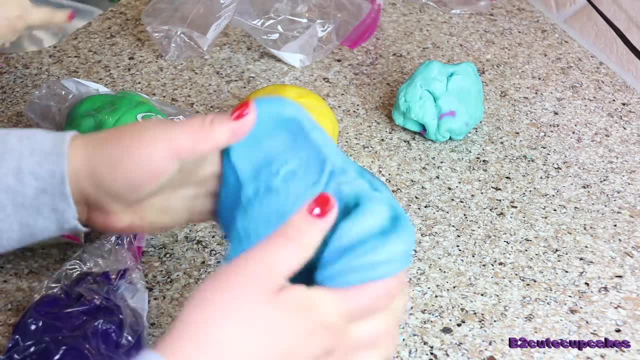 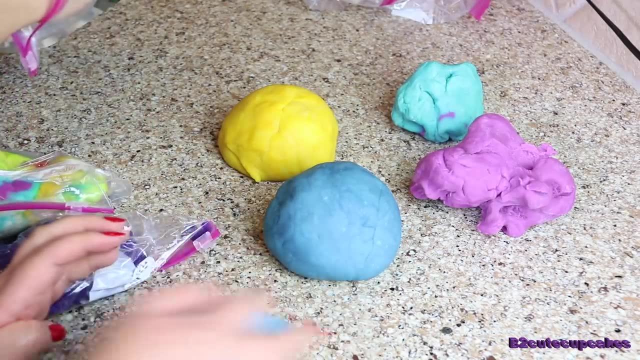 And look, The texture is still the same. It's pretty soft, It's not hard at all. You are going to discover on your own that when you make this playdoh, if you take good care of it, it's going to last you forever. 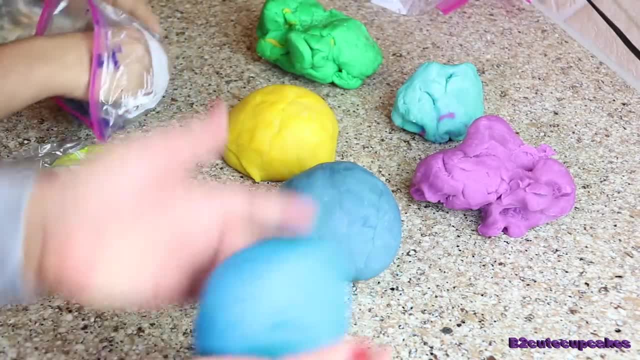 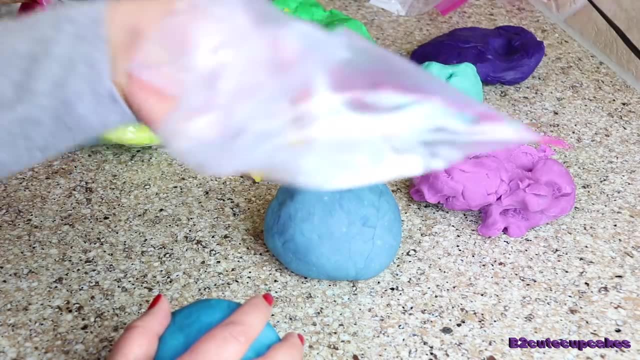 Now, don't just leave it there hanging like that, because then it's going to dry. When you finish playing, you put it on your little bag, You take all the air out and then you seal it and then you place it inside one of those. 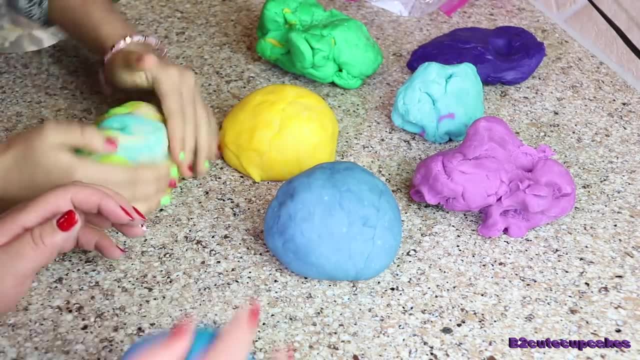 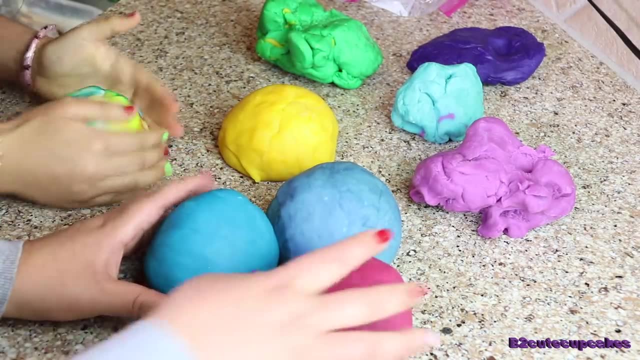 bags that they keep you in the market, in the supermarket, And then you leave it in a dark place and you see it's going to last you forever. Look, All of this playdoh is the one we make before, And look. 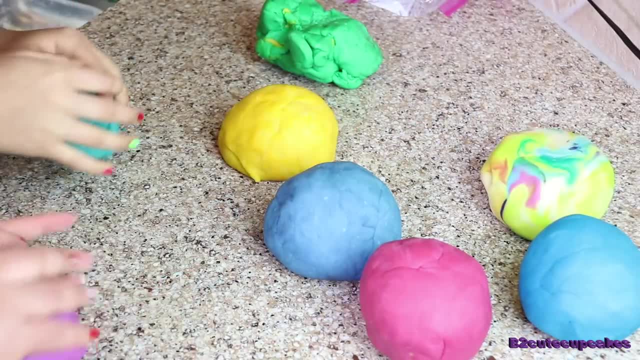 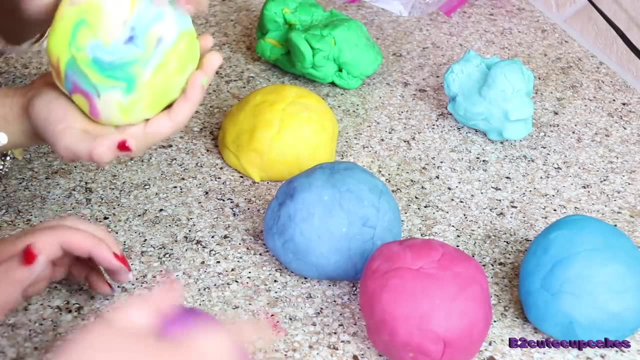 Still really, really soft. Oh, show them that one. That one looks so cool. Look at that one. It's a rainbow. It's the one the girls use to make the playdoh challenge. In case you haven't seen the playdoh challenge, go check it out. 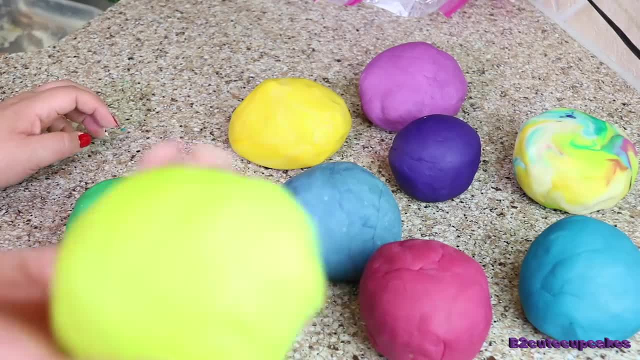 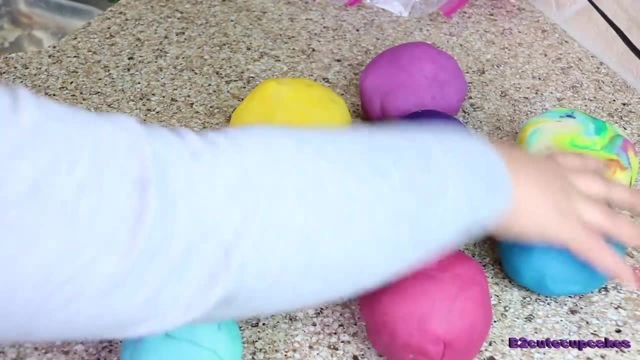 Look how cute this is. I like this color a lot Like this. this and the yellow are my favorite colors. Well, I actually like this one. Never mind, I like them all. Okay, cupcakes, If you want just white playdoh, just don't put any food coloring in it. 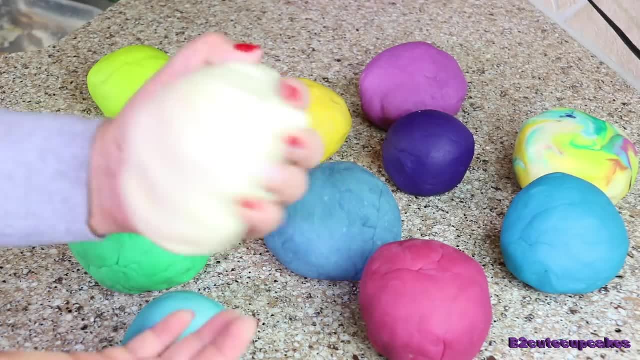 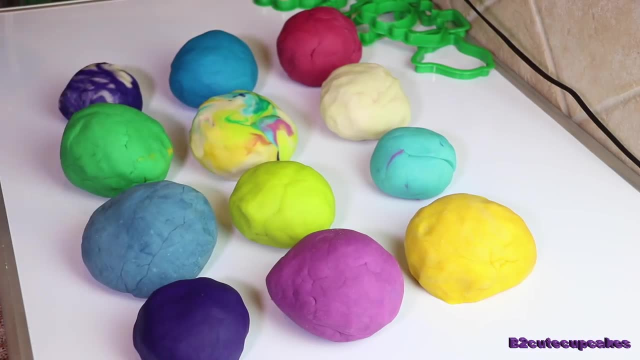 Just leave the dough as it was at the beginning and you'll have white playdoh- Okay, cupcakes. So here's all the colors we have. We actually have more, but these are the ones we're going to play with today. So we have blue, red, blue. 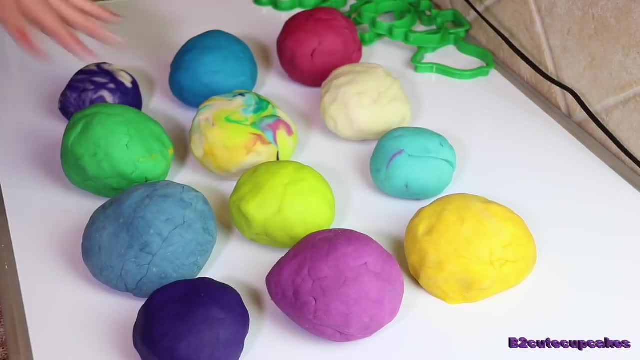 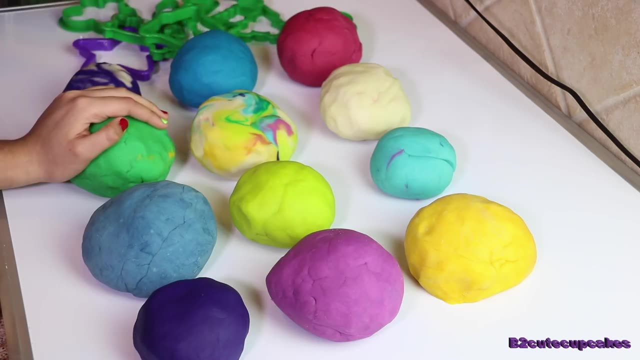 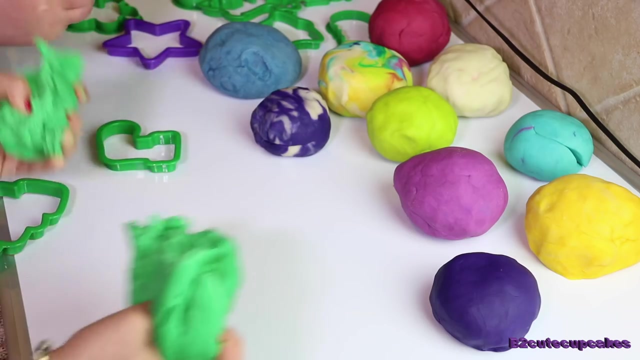 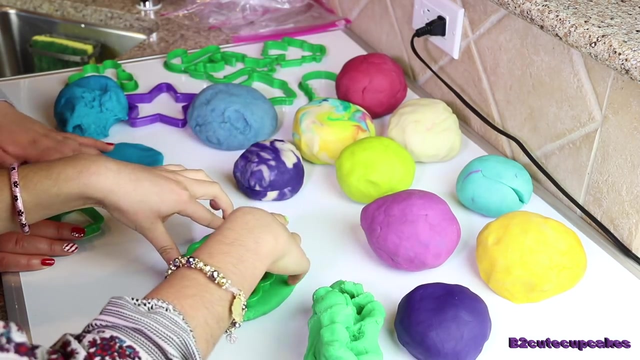 White, blue, yellow, purple, different tones of green. And here we have a lot of Christmas molds And you know, Vy says she wants to play with them. So what do you want to make? Christmas tree, Christmas tree, I'll make the stocking and I'm going to make it blue. 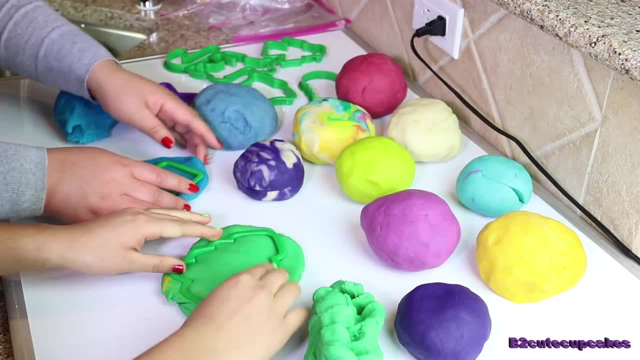 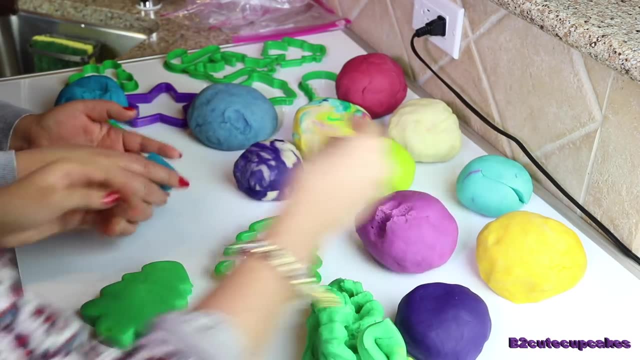 All right. So I hope you guys can see what we're doing here. Oh, I like your Christmas tree. It looks cute. Ornaments, Ornaments, All right. So here's that. Now I'm going to make a reindeer. 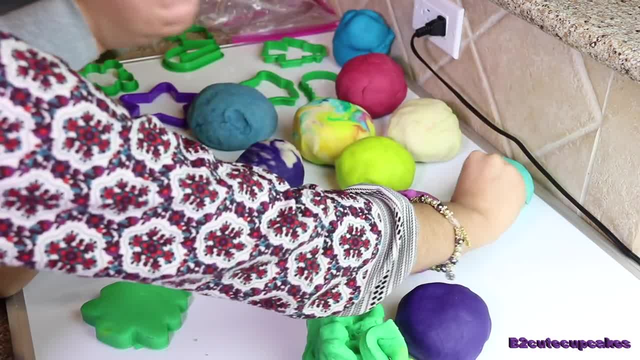 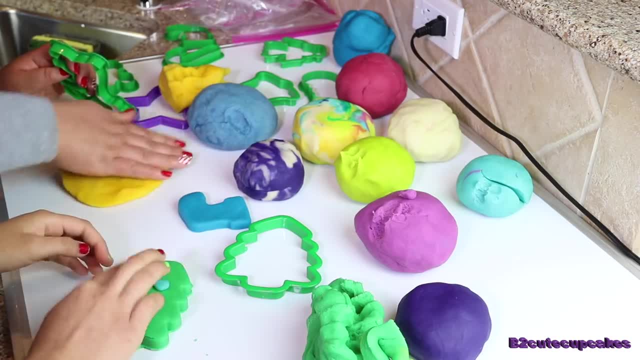 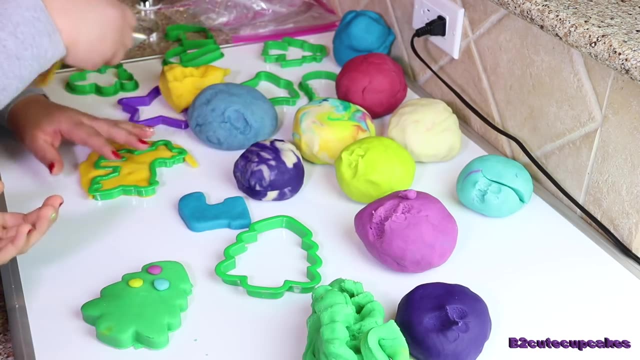 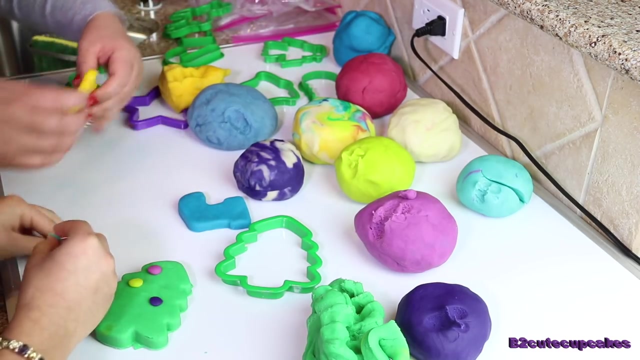 And I'm going to make it yellow. This is the one we just made, So it looks so soft and it's still warm. Okay, Let's cut, Cut, Cut, Move the excess. Oh, what do you think about my reindeer? 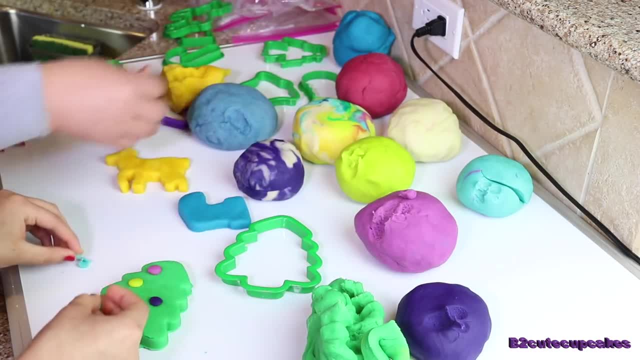 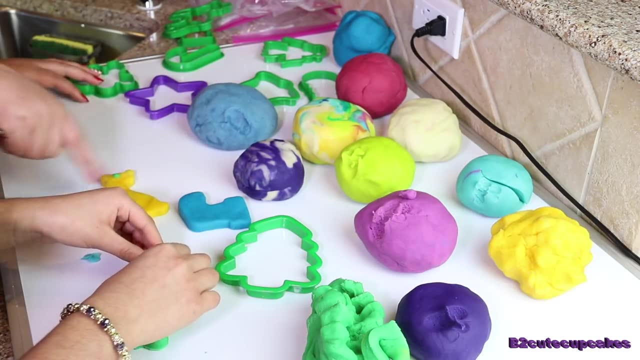 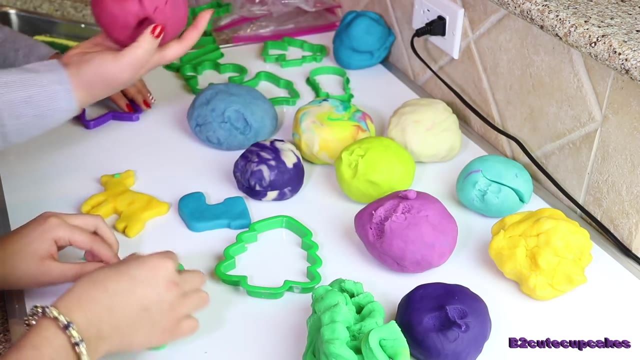 It's cute. I'm just going to use a little bit of green. Put an eye right there, Ta-da. So I already used the two colors we made today. Now I'm going to make this giant star. I'm going to make it red. 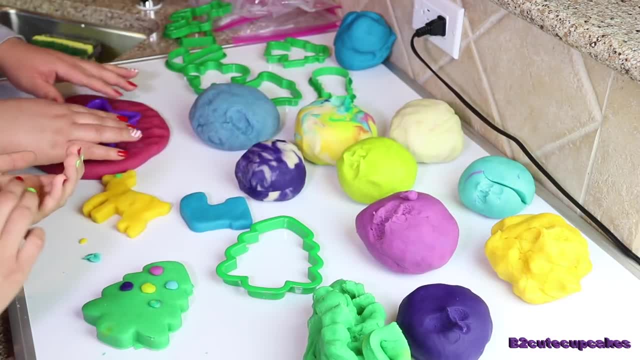 I'm going to cut it. I'm going to make it blue. I'm going to add some color. I'm going to add some more purple. I'm going to add some more pink. I'm going to add some more purple. I'm going to add some more yellow. 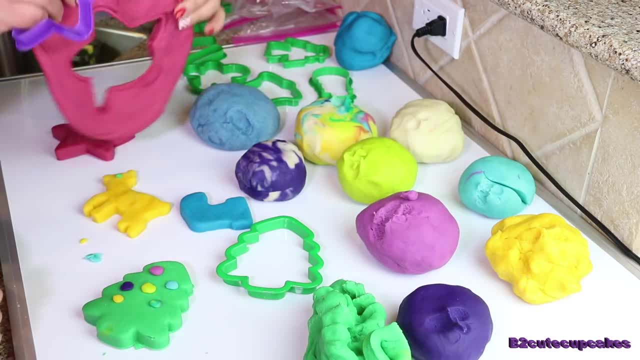 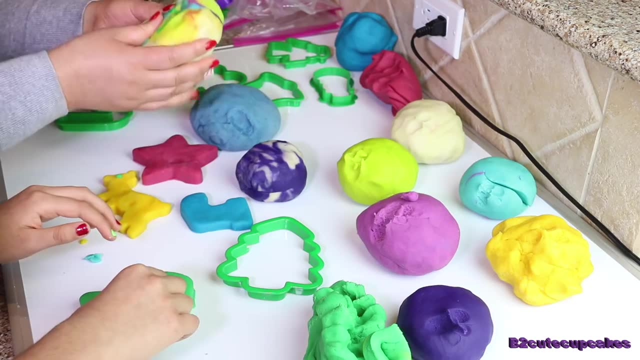 I'm going to add some more red. Okay, Let's cut There. Look at this, Hi. Now let's make a candy cane- That one I'm going to make with this rainbow play-doh. It's going to look so cute. 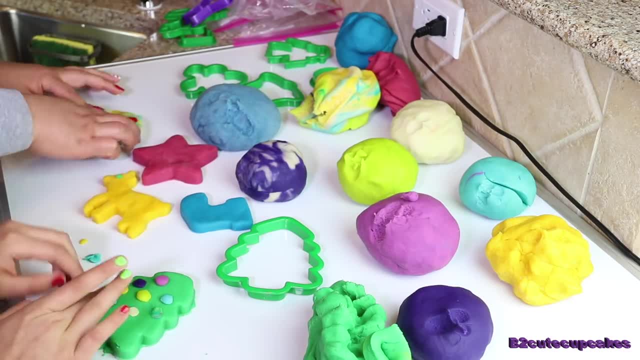 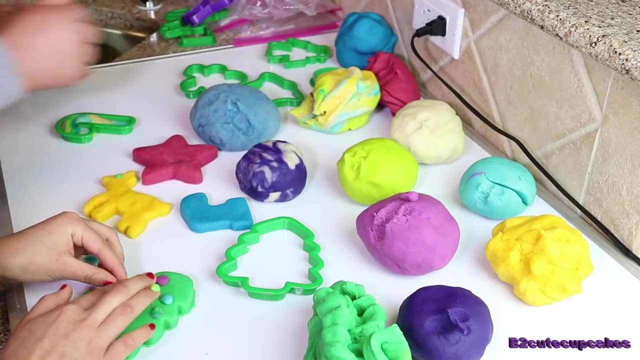 Sorry cut, Sorry cut. That's not how you do it. That's how you do it. Why don't you cut it? Sorry, Cupcake Bee can't really talk today because her throat really hurts. so, yeah, she's sick. 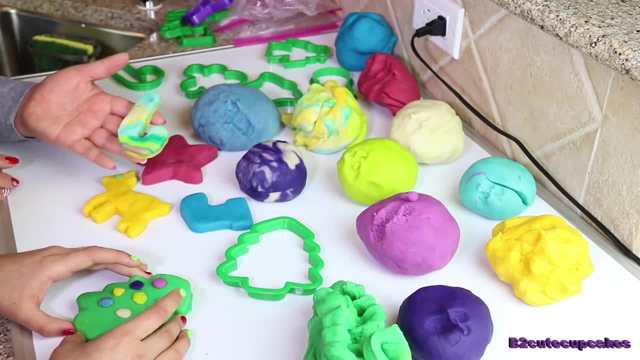 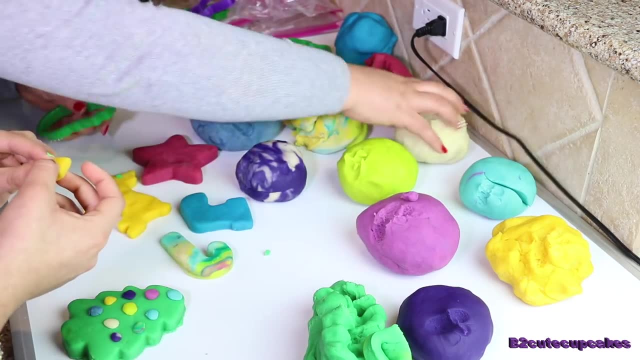 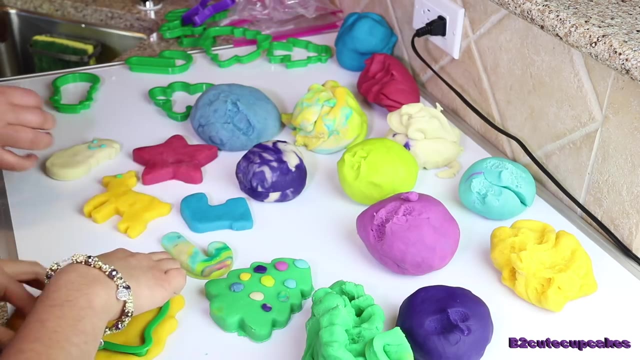 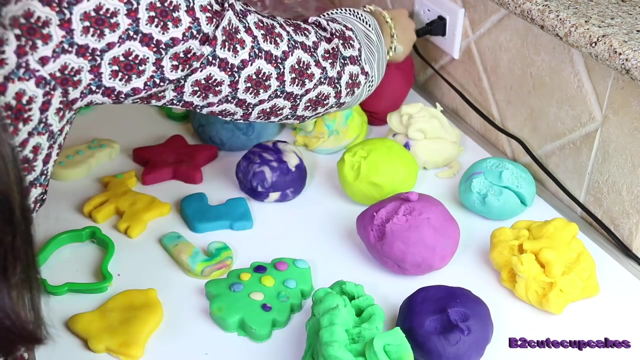 Look at my candy cane. Oh, that's cute. It's rainbow. Okay, now we have a snowman, so this one, I'm just going to make it white. Voila, Now Bee's making a bell. There there's my snowman.